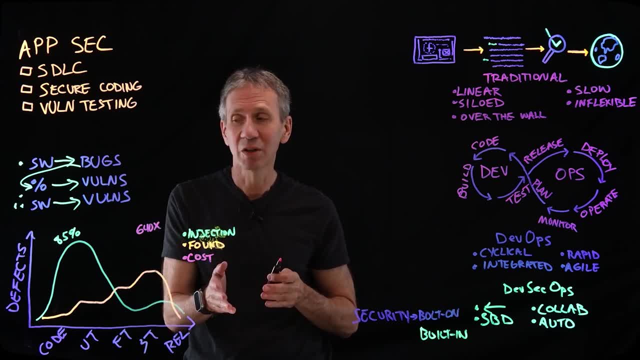 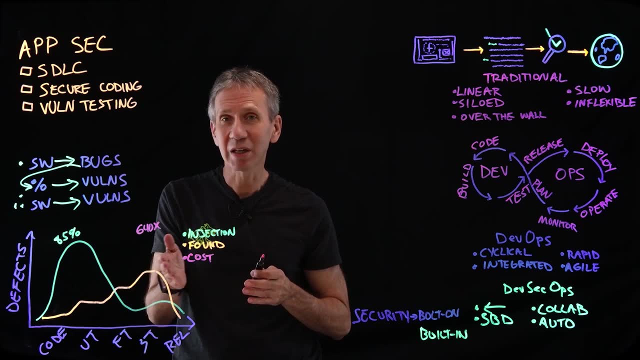 that's the green curve. But that's when they're introduced. When are they found? Well, they're found as we kind of move along. this process During the coding phase is when we're introducing them but not finding them. In the testing phase, we're finding them And then 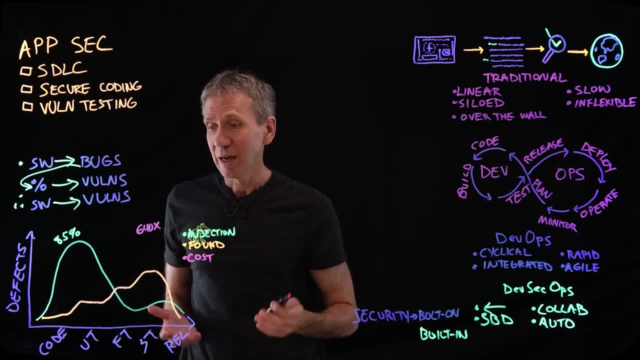 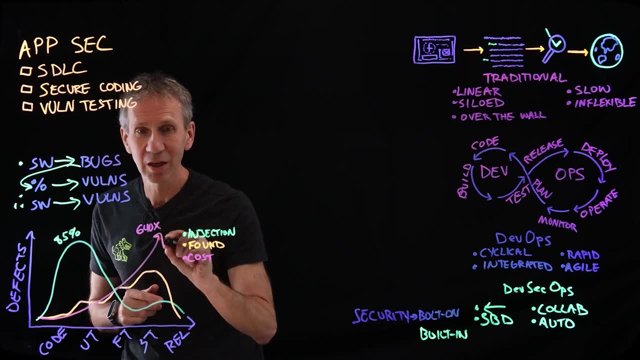 hopefully, when we get to the real world, we don't find quite so many. Now, the interesting thing about all of this is the cost. How does the cost go? Well, it turns out. cost goes about like this: where we go from 1x. 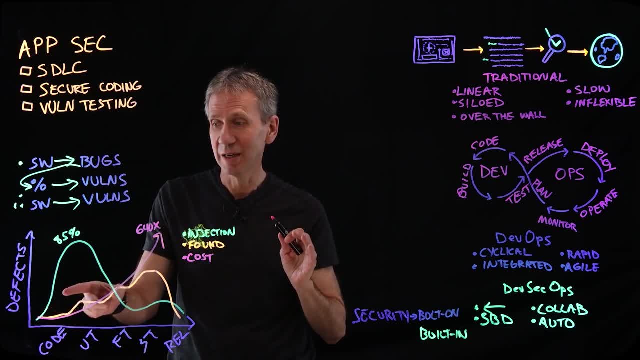 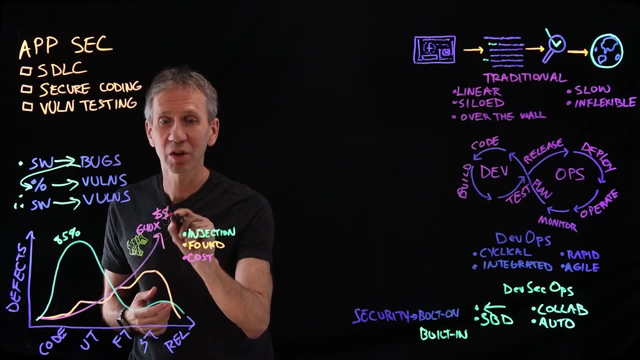 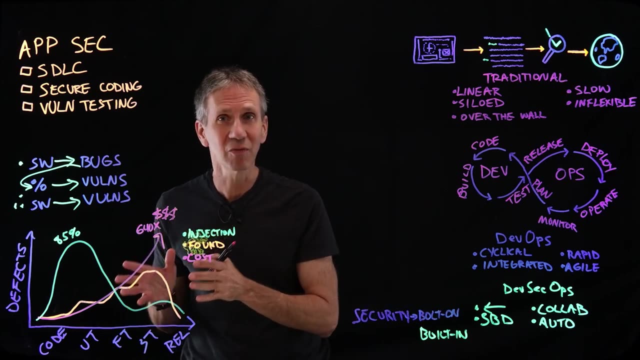 as the whatever you want to base the cost to fix a bug down here in the coding phase to, in some cases, 640x. It is vastly more expensive to fix a vulnerability once it's in the field than it is to catch it early. So there's a huge incentive for us to get this right and get it. 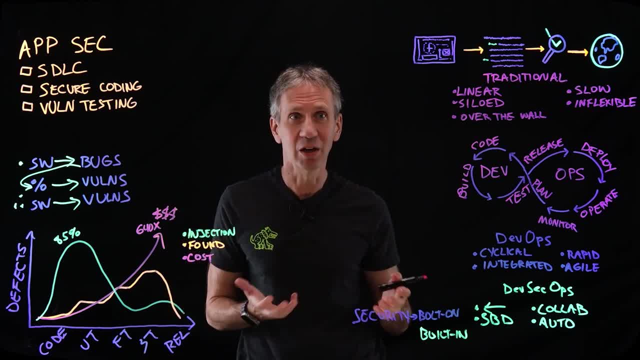 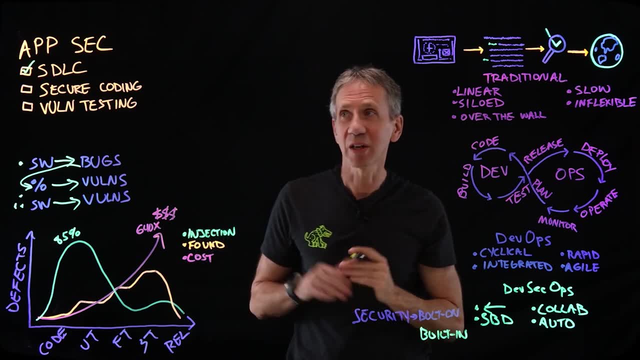 early Now. what can we do, then, in order to get this done more quickly? Well, let's take a look- We're going to take a look, by the way- at this software development life cycle That's the SDLC, And traditionally this is how it's been done. We have some design phase here. 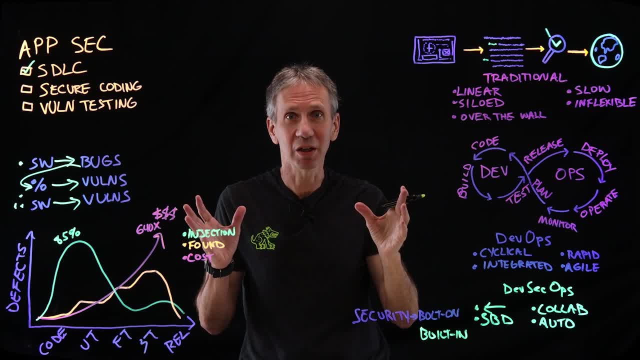 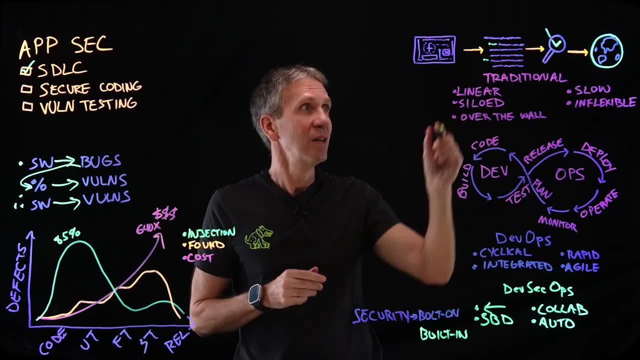 where we're going to figure out in general what we're going to do in this particular application, And then we're going to move to a coding phase. We're going to write the application itself, Then we're going to go to some sort of testing phase And then, ultimately, we release it to the world. 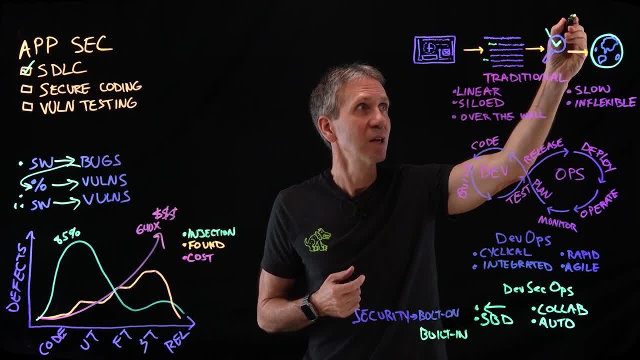 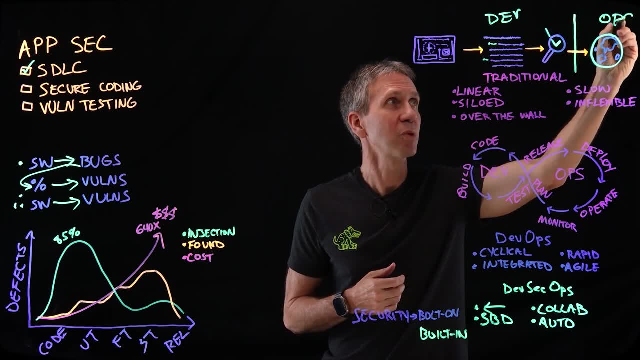 and put it in production. Now what has traditionally happened is there's a big line separating these two, where this is the dev part of the process and this is the ops part of the process. This is where we're developing, This is where we're. 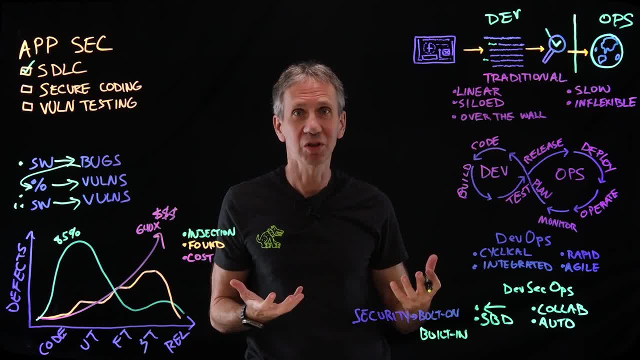 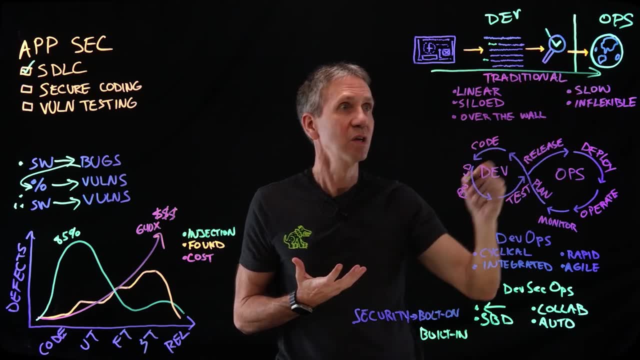 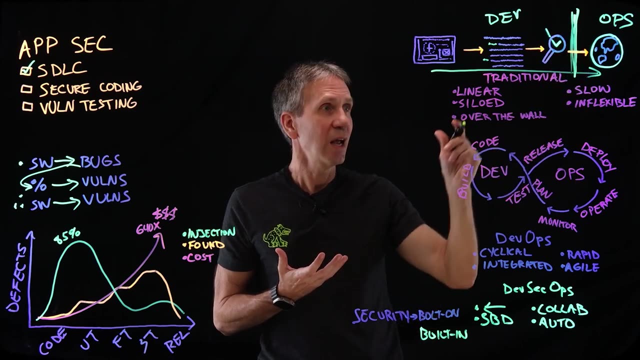 releasing and then just operating it and running it in a continuous state. The problem with this traditional approach is that it's very linear. You can see how this process goes. It's also very siloed. This line right here could be very thick in some organizations And it kind of leads to 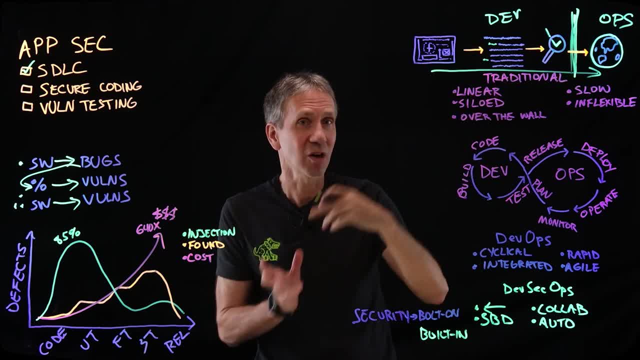 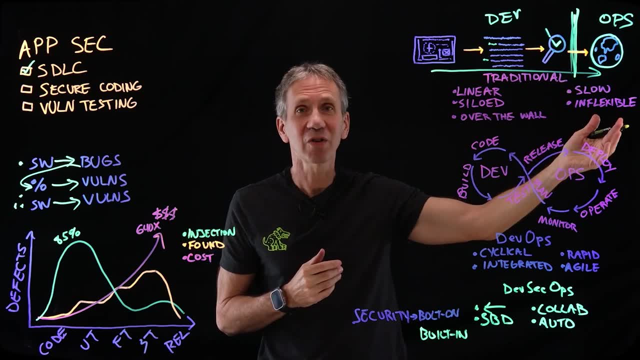 this sort of over the wall mentality. I'm going to write the code and then I'm going to throw it over here, And so there's not a lot of communication happening here. It can be a slow process and it's fairly inflexible. And, by the way, I'm going to suggest to you we didn't really 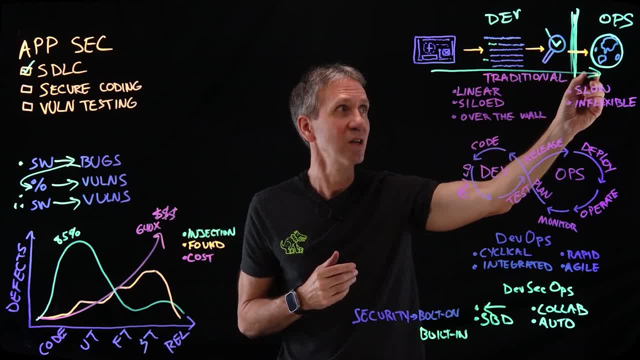 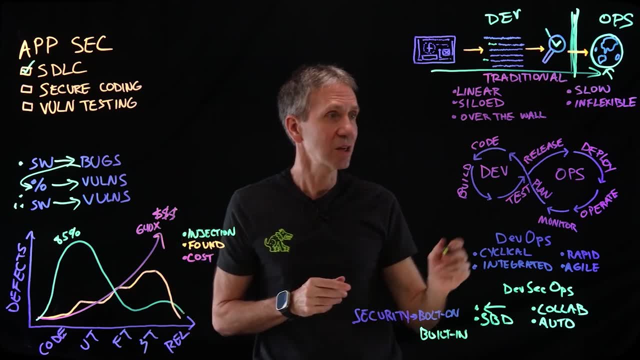 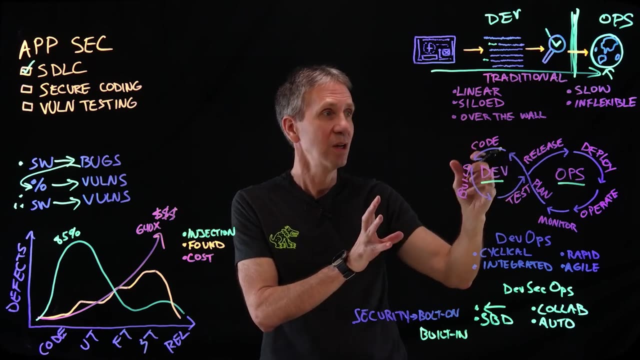 introduce security very early in this process. Very often security gets introduced out here, and that's a problem. Now, a more modern approach to this is this thing called DevOps. So here we take the two processes: dev, where we're building the code, then we're releasing it, we're deploying. 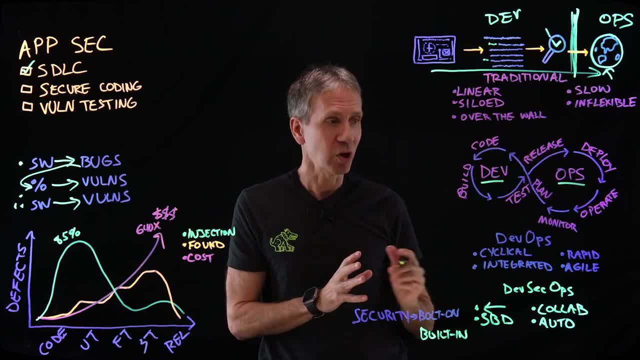 it, we're operating it and we're feeding it to the world, And then we're building the code, and then we're feeding back With a DevOps process. now what we've got is a cyclical type of situation. This 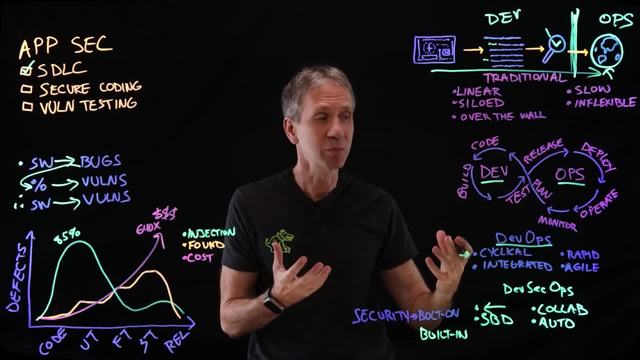 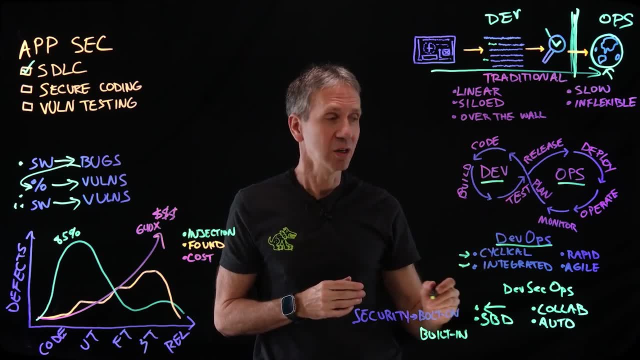 thing doubles back on itself. There's a feedback loop of continuous improvement. There's no over the wall. There's no us versus them. It's an integrated process. It's much more rapid and it's designed for agility. So this is a much more flexible kind of capability. 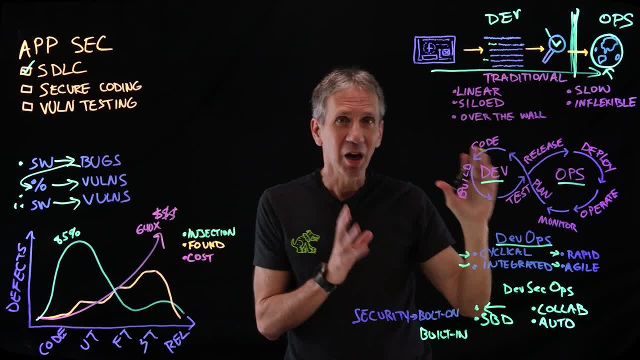 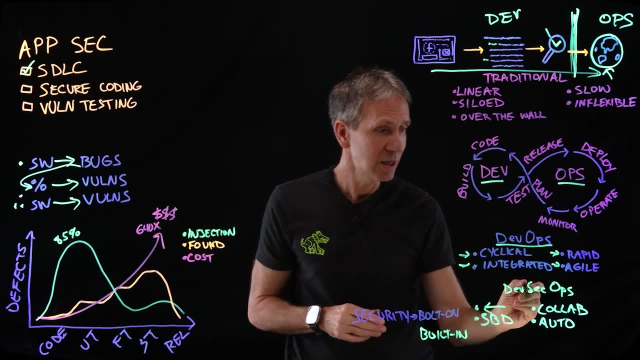 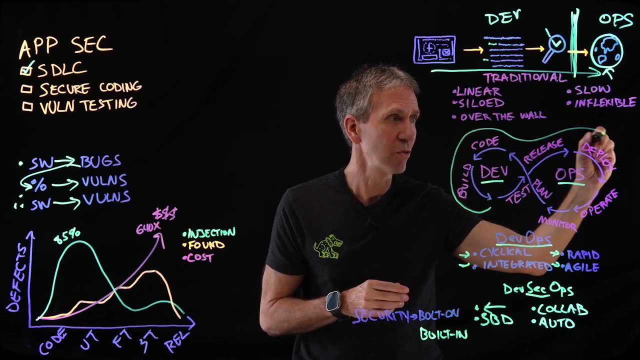 moving away from this traditional linear approach. But again, we haven't really addressed the security here, And so what more modern approaches have done is introduce this notion of DevSecOps, where now we're going to basically bathe or encompass the whole thing in a security. 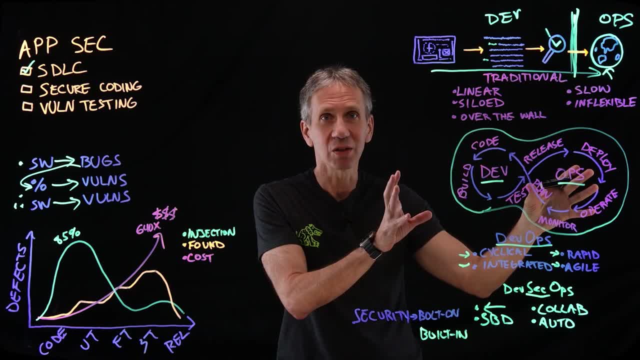 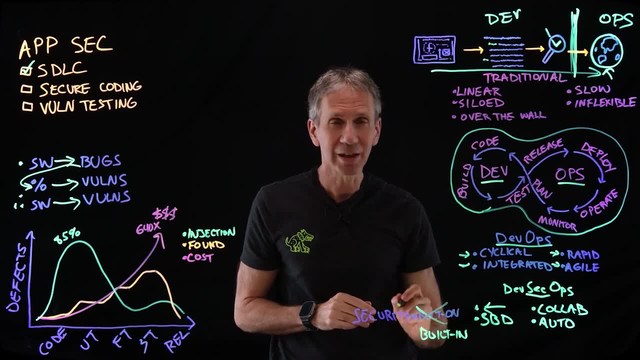 layer. We're going to put security at every one of these phases. We don't want this to be something that we wait to the end. Security can't be a bolt-on That is not going to be effective. We need security to be built in and looked at at every one of these phases. 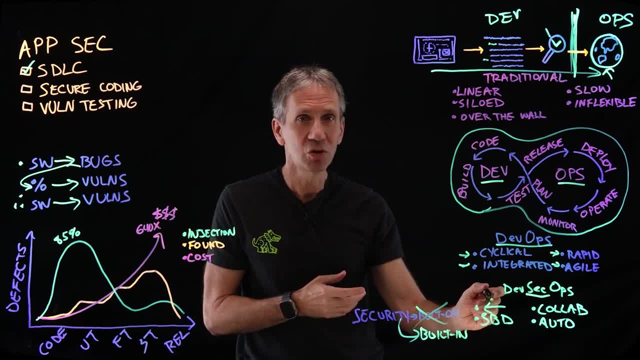 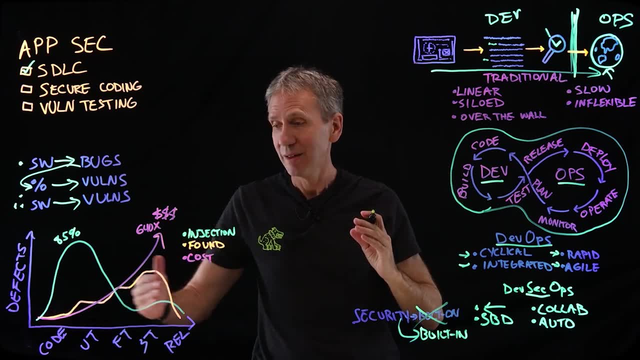 So, for instance, with a DevSecOps approach, we're going to do what is referred to as shift left thinking, That's, if you were thinking of this in a linear phase or thinking of it this way, Then we're going to put security not just here, We're going to introduce security at each one of these. 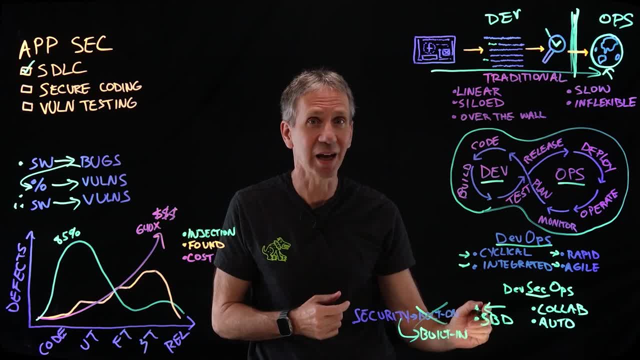 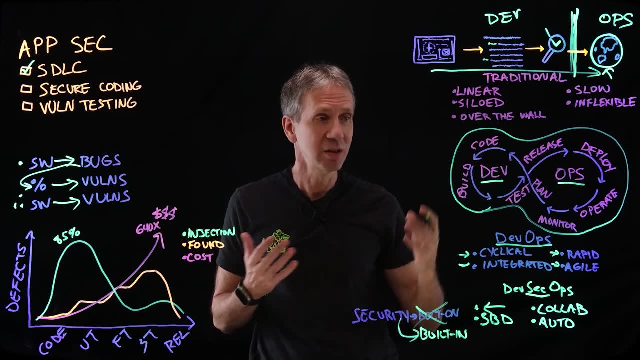 phases. We're going to do security by design. We're going to design the system so that it stands up and it's resilient to attack from the first, not again as a bolt-on. Then we're going to create collaboration among what we call the business teams. 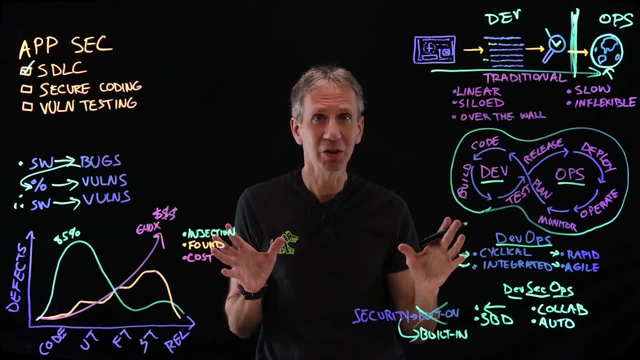 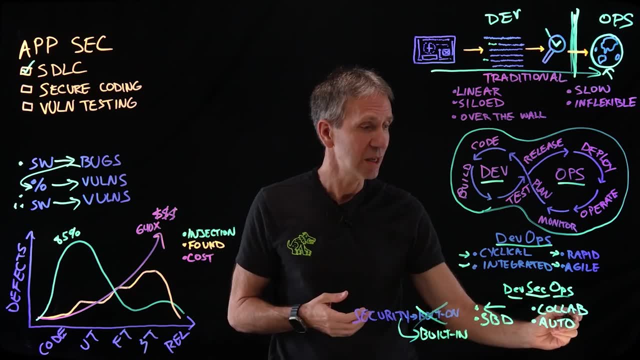 have been traditionally three different groups that maybe didn't always talk together, but with devsecops we have it all working together, with a lot of collaboration, a lot of feedback, and then ultimately try to leverage a lot of automation. i'll talk about that in terms of tooling a little. 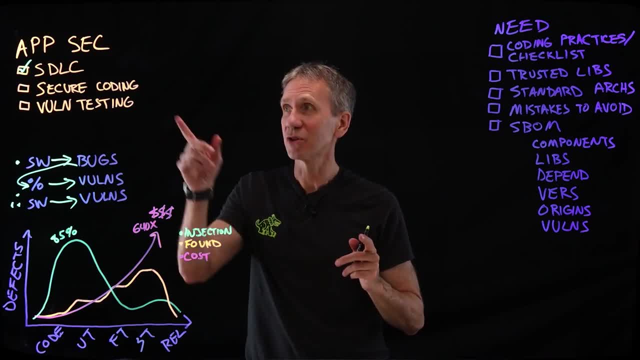 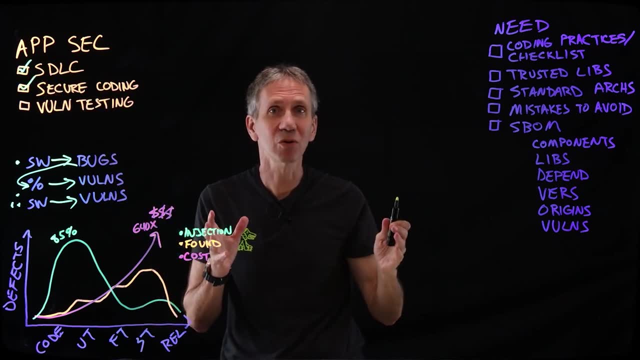 bit later in the video. okay, now we've covered the software development life cycle. next we're going to take a look at secure coding practices and things like that. what do we need in order to write secure code if we're going to shift security left all the way to the coding, maybe even design? 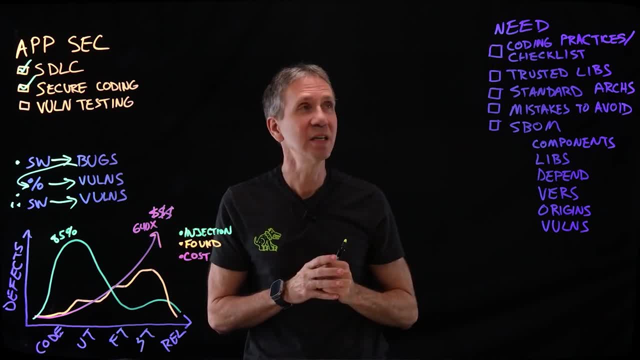 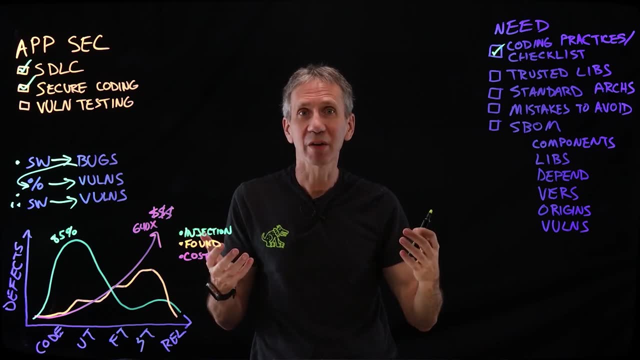 phase, but we're going to focus on the coding part right here. what are my needs? well, one thing i need is a list of secure coding practices. this is a prescriptive way of saying. this is how we should go about writing certain code. there are certain things that we need to do, for instance, validate. 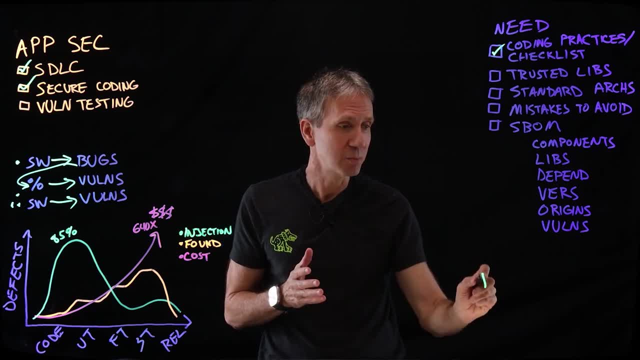 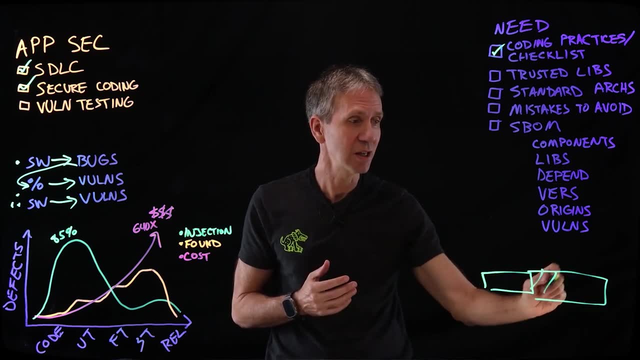 inputs. we need to make sure that if a buffer has been allocated for this size for input, they That when someone sends me something it's not this big, because then in that case it could be overriding memory. We call this a buffer overflow, So that's a type of condition that's been around for a long time. 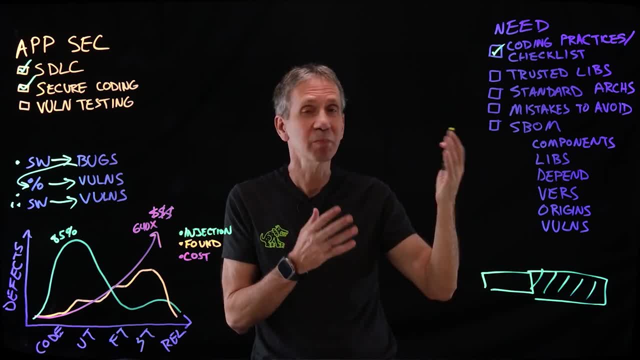 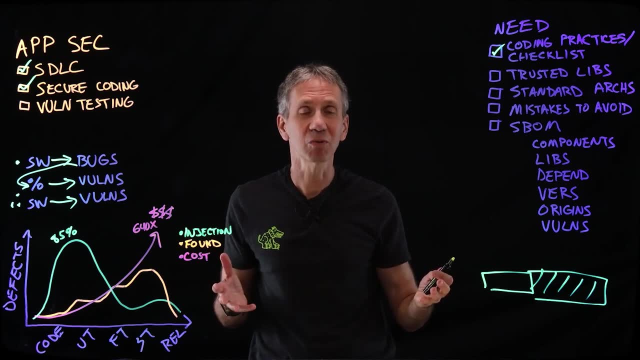 If we don't do all the input checking, we could have problems. We need to specify how we would do authentication. What are some of the other ways that we would use cryptography, What kinds of error handling routines? So it's basically a way of saying: have we checked off all of these things? 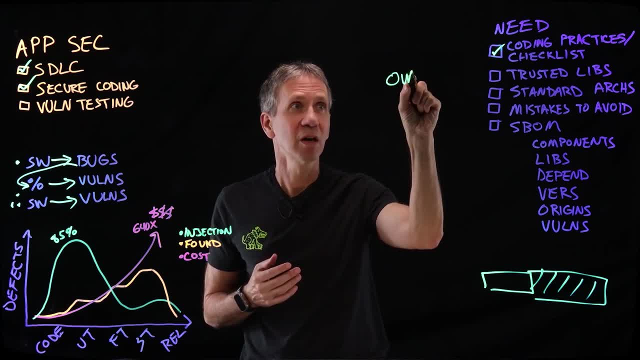 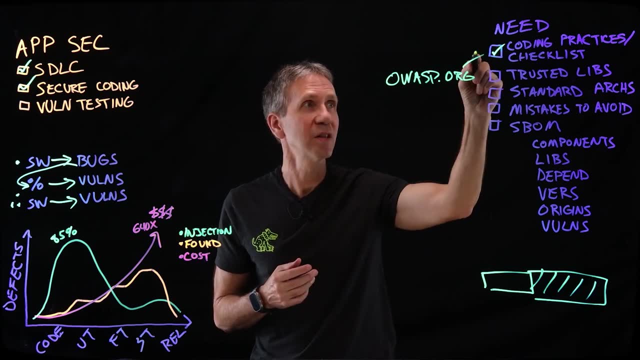 Have we done them all correctly? Well, there's a great resource here. It's called OWASPorg, And at this website what you'll find is they have a list of secure coding practices. They have a very good document that is kind of an industry standard that a lot of people 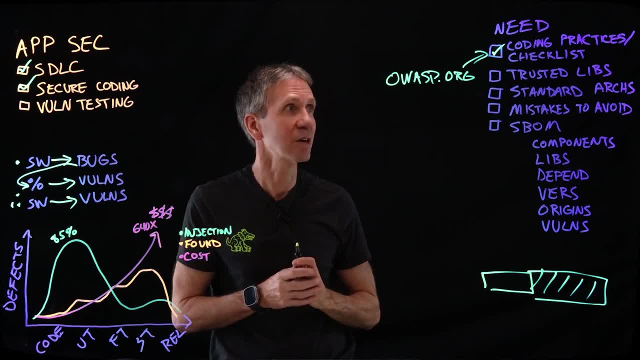 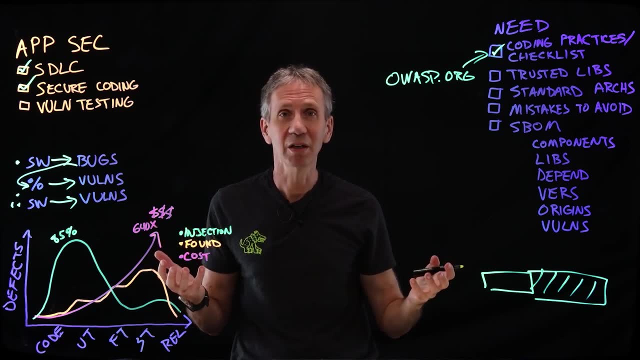 use in this, So I would reference that. you take a look there: Trusted libraries. Everyone doesn't write all their code from scratch anymore, because there's just too much that needs to be done, So, as a result, we end up relying on code that's been written by other people. 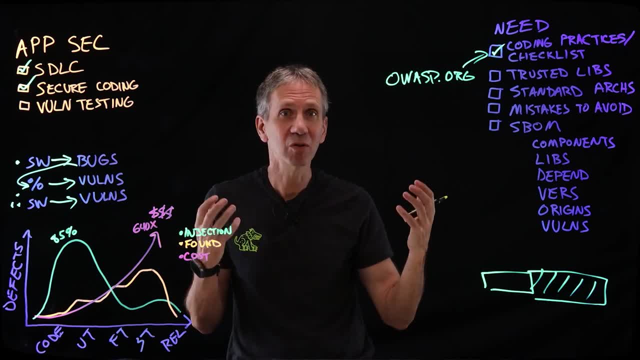 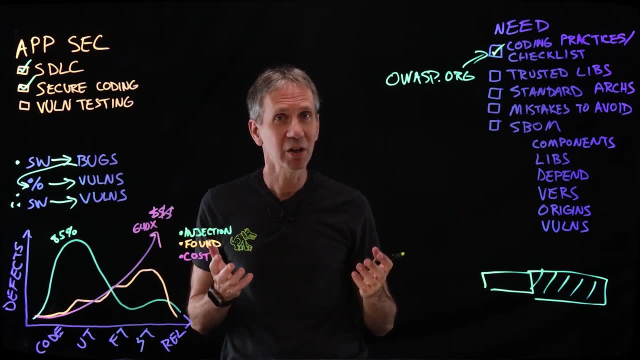 It might be open source, It might be proprietary, But we're going to use this in our code as well, or make calls to it and leverage it. There's a lot of sources that are out there, but not all of them are trustworthy. 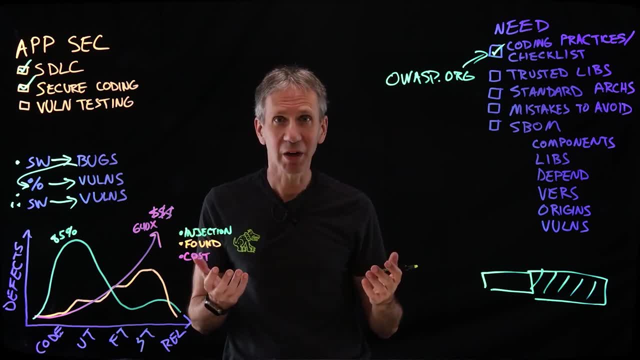 And even the trustworthy ones need to be looked at with a certain amount of skepticism and a certain amount of inspection. So trusted libraries are an important thing here as well, And if you want to see what can happen even with a trusted library, go look up something. 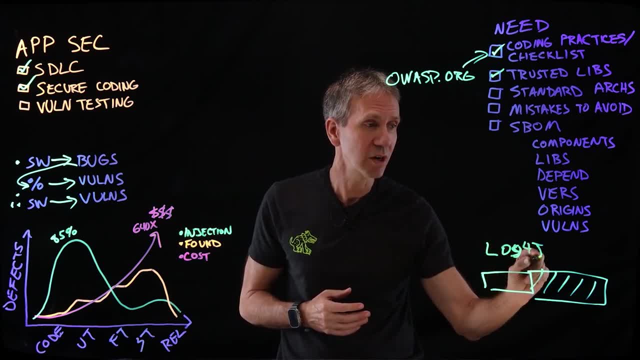 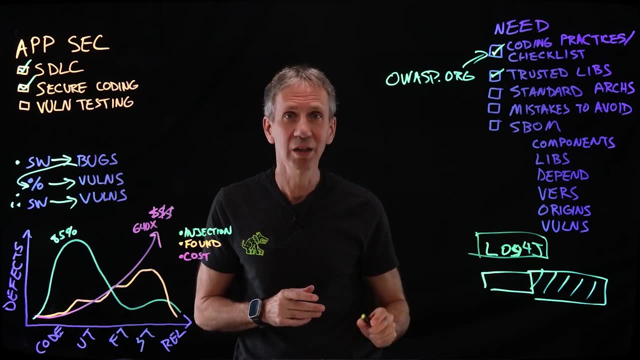 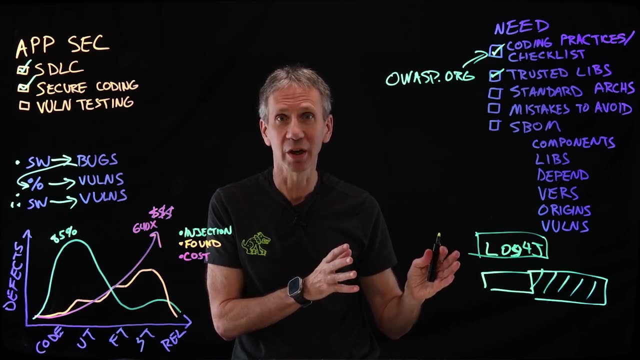 called Log4j. This is a very well-known vulnerability. It's a vulnerability that affected tons and tons of systems because everyone was using this routine, which was a common, trusted routine from trusted sources, and yet it had a vulnerability in it that an attacker could exploit. 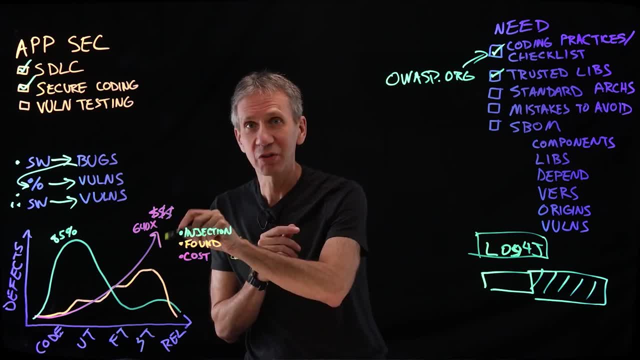 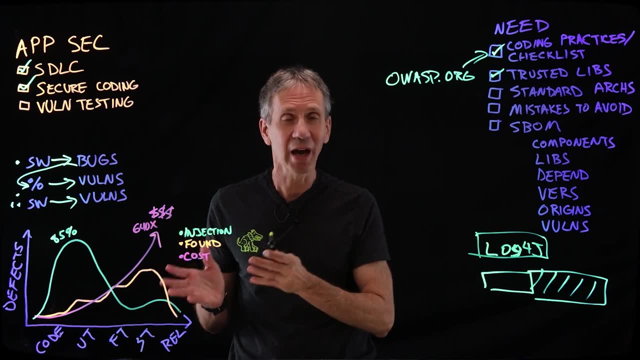 And those vulnerabilities were discovered- guess what? over here, in this phase, right when it was the most expensive after it had been released. So again, we want to try to eliminate that, or at least find it much earlier in the process, if we can. 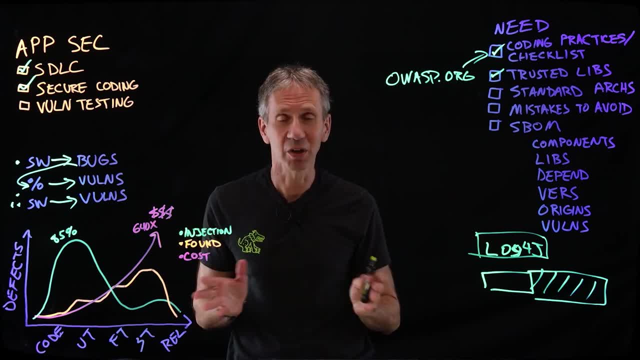 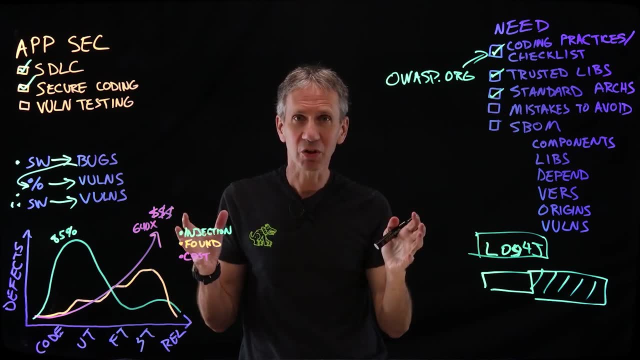 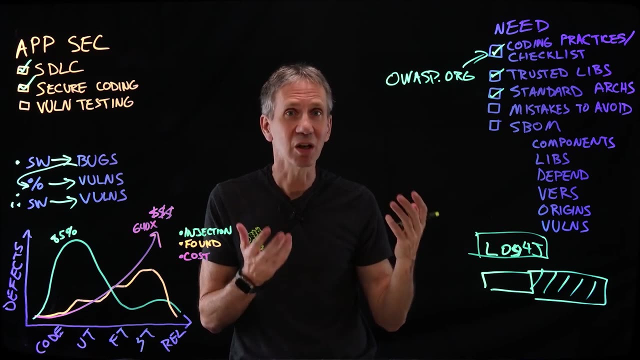 And using trusted sources At least helps. It doesn't eliminate the risk, but it helps Standard architectures. I want to have spelled out that when we're going to do a certain approach, this is how the system should look. So we want to spell out in advance what those would look like. 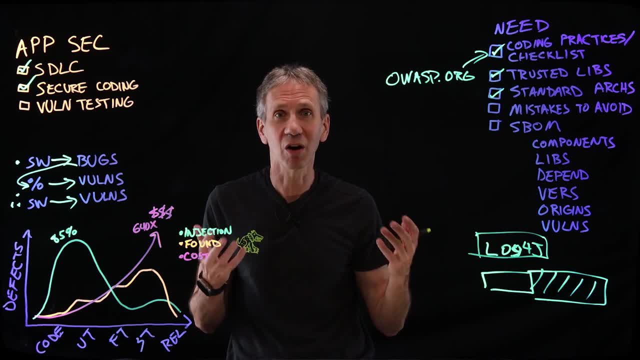 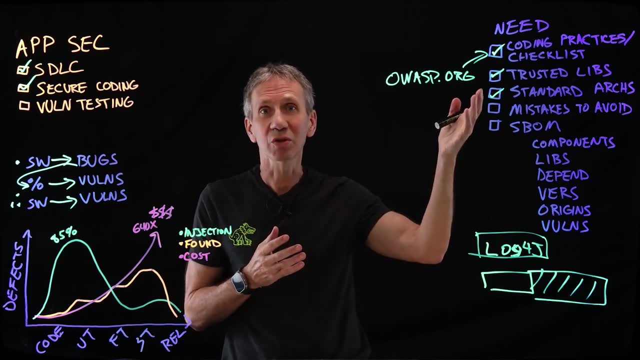 There's a lot of different sources for that. IBM has an application security architecture reference website that you can take a look at and we'll reference here Also. there are other sources, but you want to be able to spell this out for your whole organization. 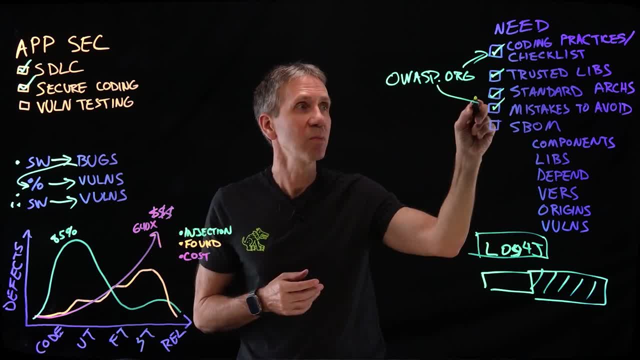 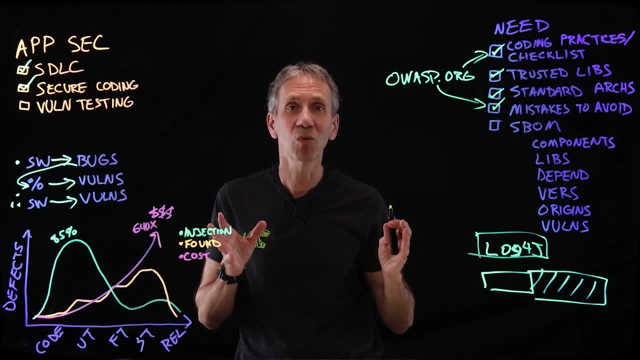 So that they can see that Mistakes to avoid Again. we're going to go back to our friends at OWASP. They have a thing called the OWASP top 10 list And what's really interesting in this is they're showing what are the top 10 vulnerabilities. 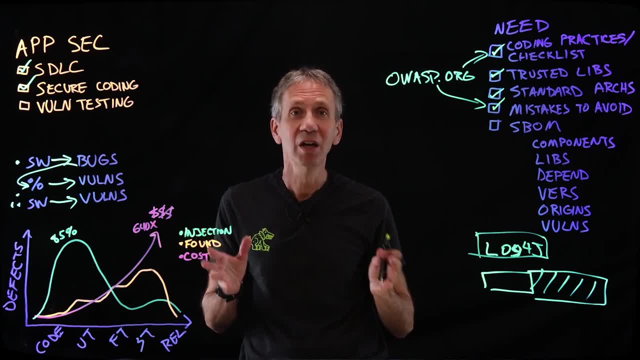 that we keep seeing And it's very interesting to look at this over time. Look back in 2017, what were the top 10? and look now and the more recent one, 2021.. And what you'll find is there been a little bit of shifting here, but unfortunately it's. 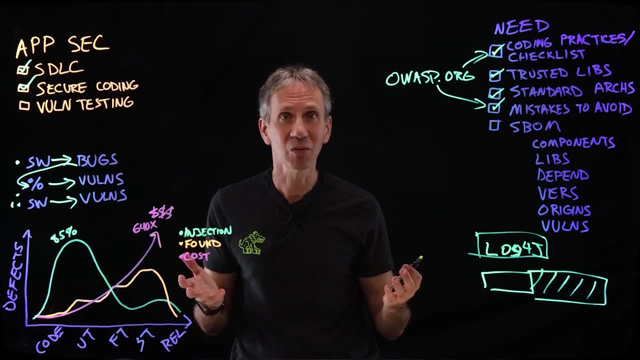 sort of the same list, Which means we're not getting better. We're not making these defects extinct, We're just kind of shuffling the order a little bit. But things like buffer overflows and other types of input validation errors have been around for a long time. 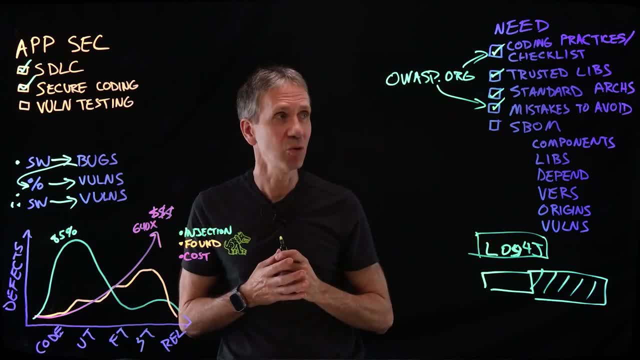 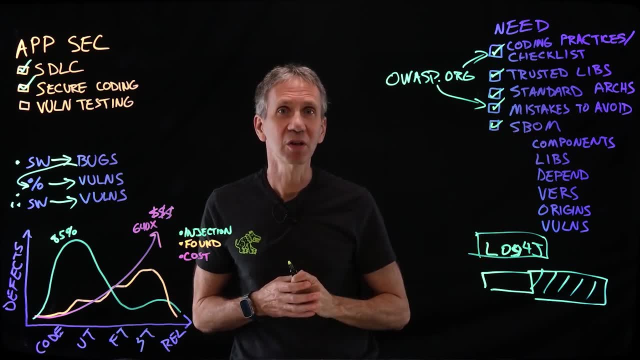 But this is a great learning resource. So, again, I refer you to OWASP. And then, finally, this notion is really starting to build some momentum, The idea of a software bill of materials That is. I want to know where everything came from. 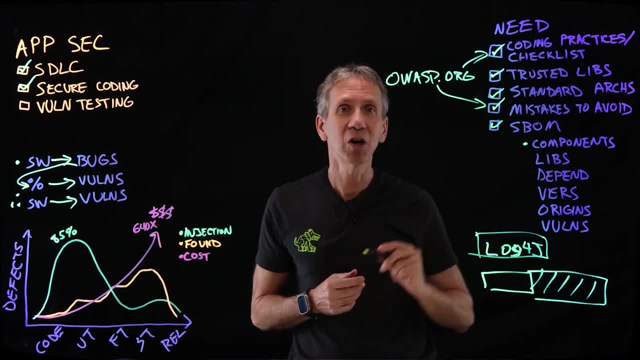 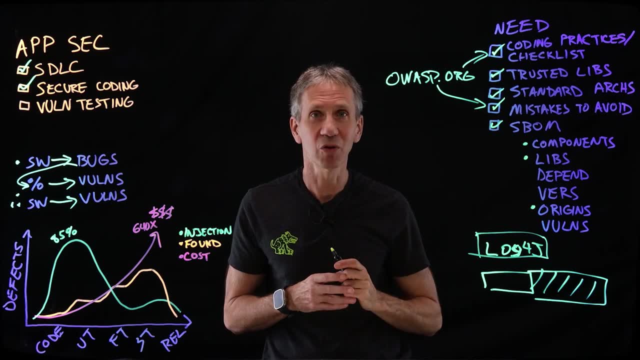 Kind of a supply chain, If you think of it this way. I want to know all the components that I'm using. I want to know where they came from, their origins, the libraries that they came from and where those are sourced. I want to know what dependencies exist amongst these different components and have those 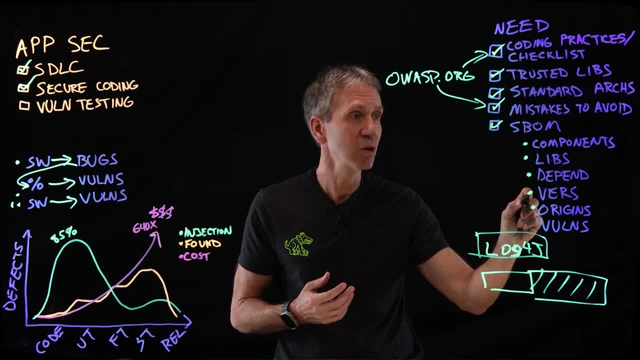 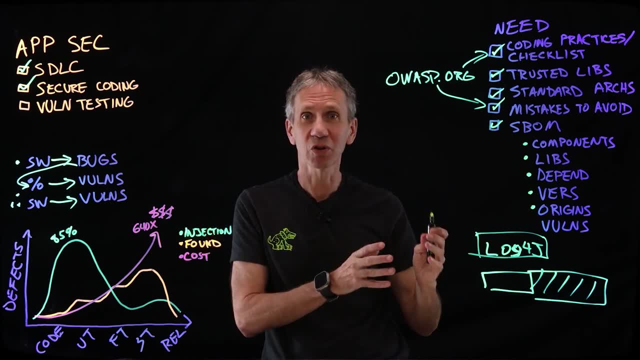 really spelled out. I don't want any surprises in that I want to know the versions of all of these that I've used across all of my different systems, And if I'm building applications, I need to know which versions are used, because those 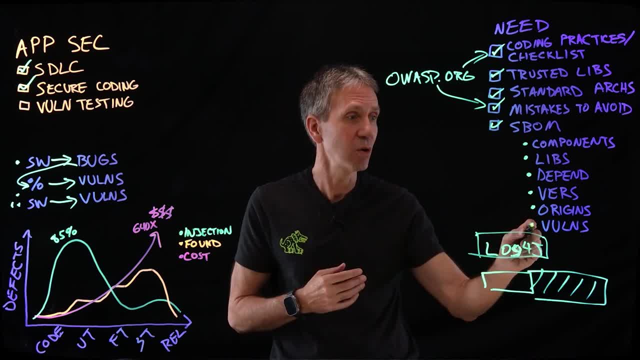 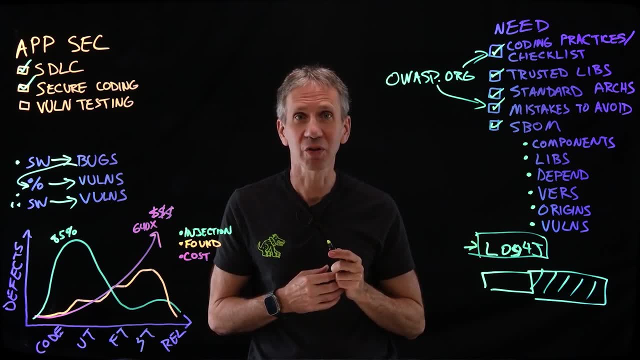 will change over time, Need to be updated And I need to be able to know what vulnerabilities might exist in those. Again, refer to log4j. Go and do a web search on that if you want to find out more about that example. 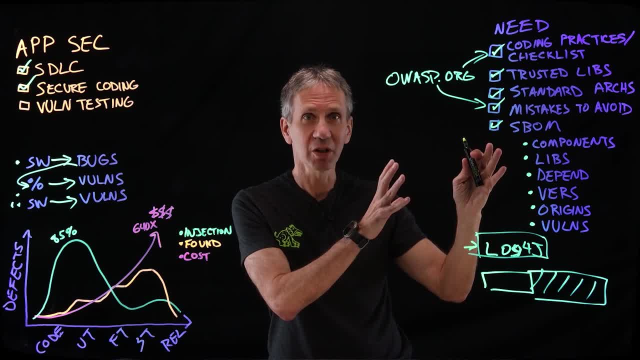 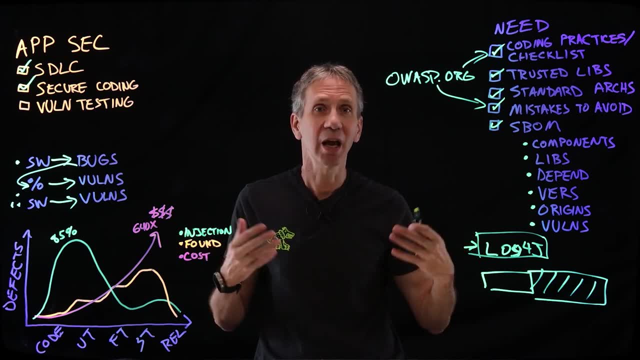 That's a good example where if we have a software bill of materials and we get hit by one of those vulnerabilities, then we have a much better idea of all the different places that we need to make changes And we can recover much more quickly and hopefully eliminate a certain amount of this cost. 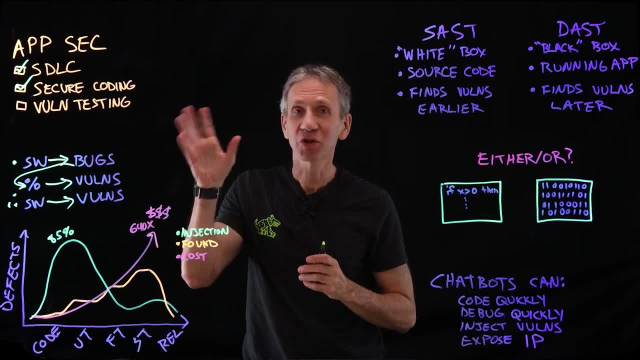 Okay, Now we've covered the software development lifecycle. We've covered the software development lifecycle, Secure coding, And we're now going to take a look at vulnerability testing. We'd like to test for security throughout the process. Remember, one of the things I mentioned in the DevSecOps process is to use more automation. 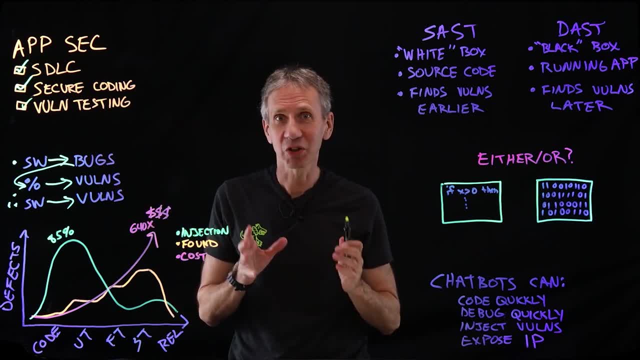 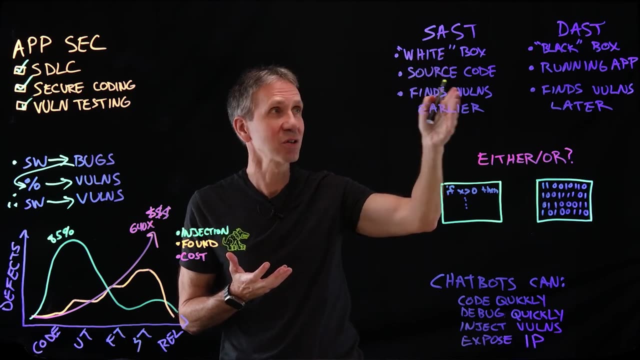 that is, use more tooling, And two major classes of those tools are static application security testing, SAST and DAST- dynamic application security testing. You figured if one was going to be static, the other is going to be dynamic, right? 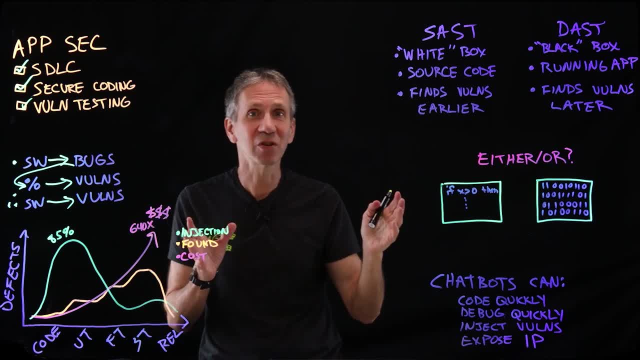 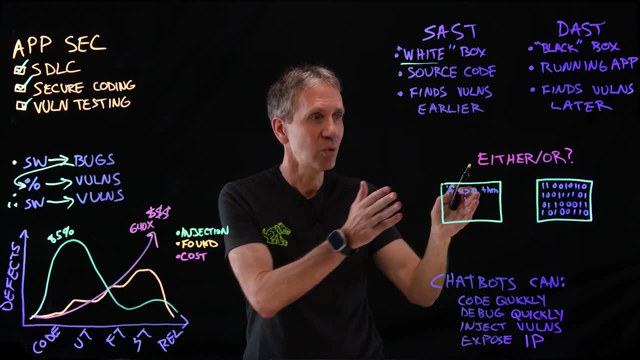 Okay, What's the difference in those two? That's a good question. what's the difference in those two? Well, the static is often referred to as white box testing. It's called that because we can look inside and feed it the source code, So it's like it's looking. 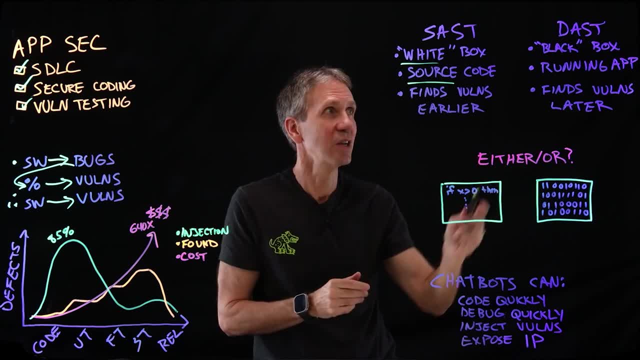 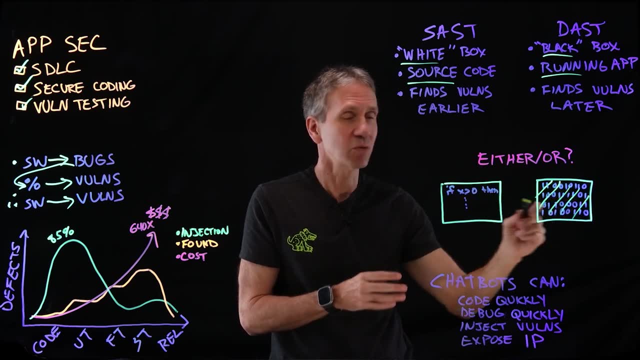 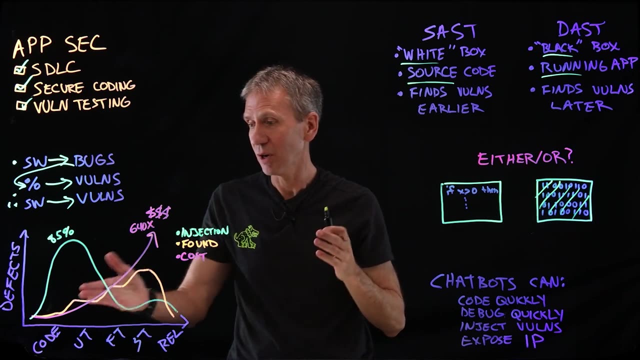 inside our code. So the box is open, in that sense, The black box dynamic. instead of giving it source code, we're actually obscuring what the source code is. It's going to look at an executable system. Think about it differently. In this case we're going to do maybe after the coding phase. 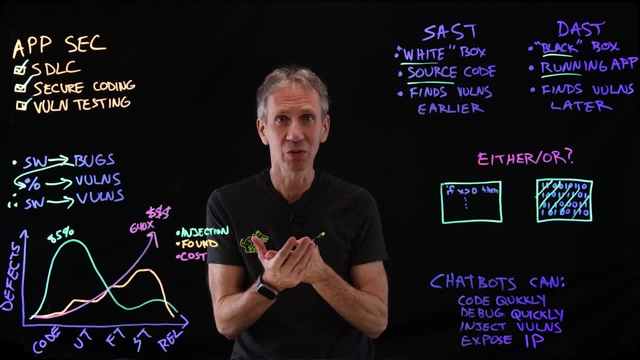 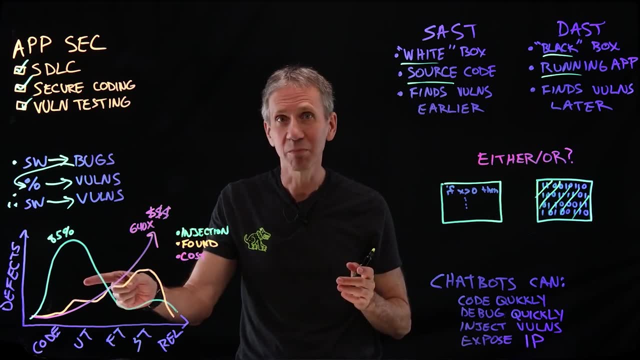 I can run one of these tools. I can feed my source code into it and it will look for vulnerabilities and tell me about those, the ones that it can identify. And the great thing about that is we're moving this much earlier. We're doing a shift left in the dev process and finding those bugs. at the earliest stage that they were introduced, therefore reducing cost. Even if I can't do it in that phase, I don't have to do it again. I can do it again. I can do it again. I can do it again. 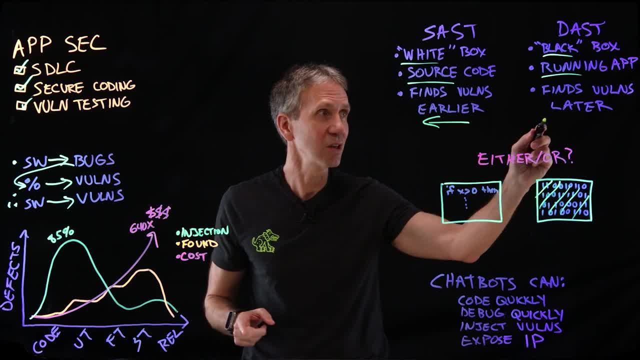 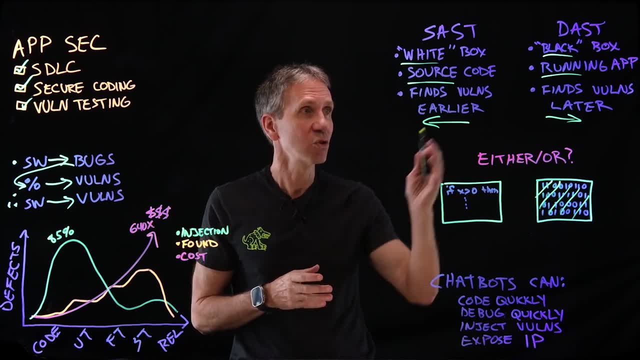 I'd at least like to catch it during one of these test phases. so it's a little bit later in the development cycle, but it's still before we hit release, when everything gets super expensive. So what I'd like to do is run both of these. In other words, it's not an either or It's really. 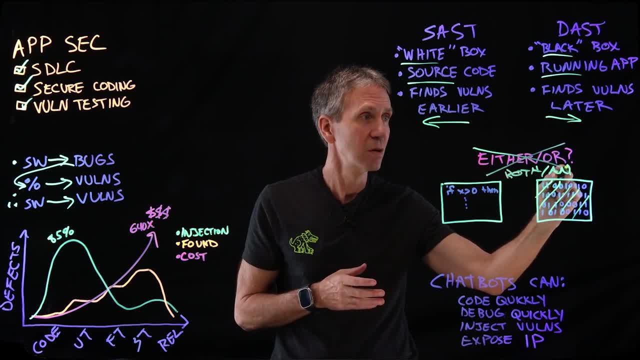 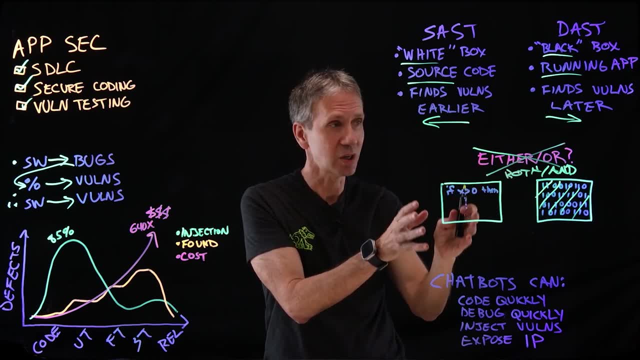 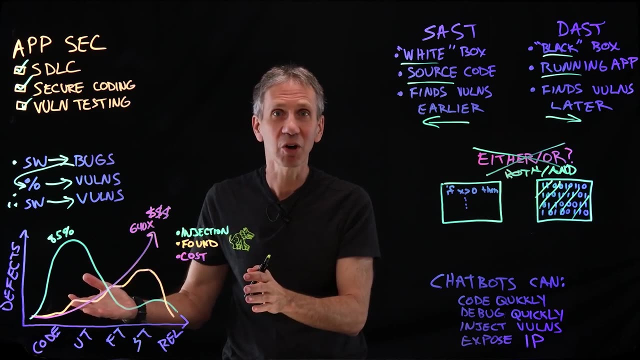 both and because there's advantages to both of these. The source code scanner will find certain types of vulnerabilities. The dynamic scanner will find other types of vulnerabilities. The warning camera will find other types. So you really need to use them both together and you use. 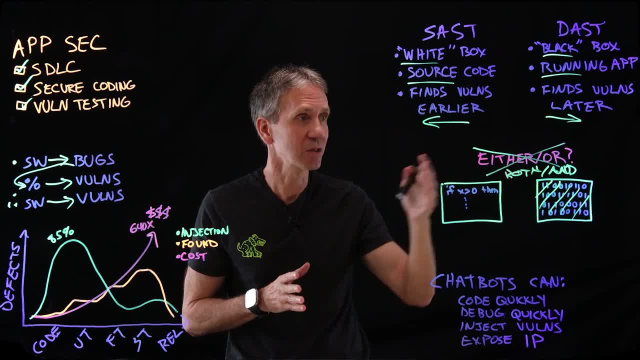 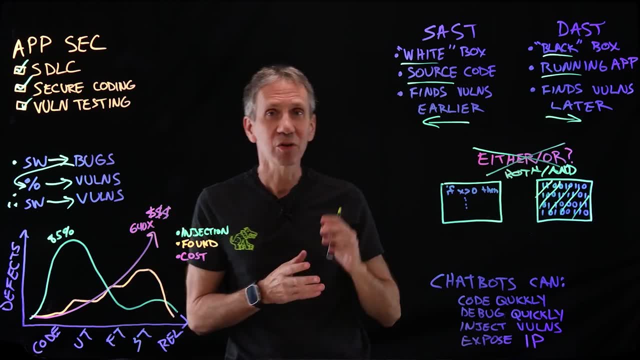 them throughout this process. And again, think about that cyclical DevSecOps process and you can see how this would fit in and how the tools now become the enabler to do better security. One other sort of tool that's being used in this space a lot for application development. it wasn't 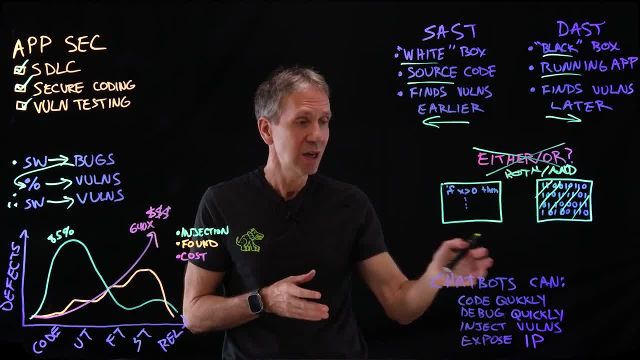 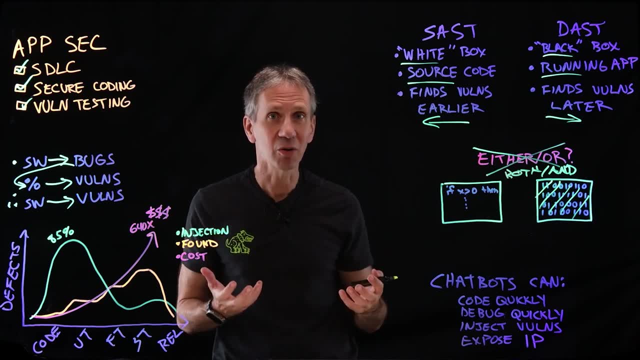 initially thought of in that context by a lot of people, but it's really becoming popular and that is chatbots, These large language models with generative capabilities. The chatbots, if you're on the capabilities, can also generate code. So a chatbot is good at generating code very quickly. 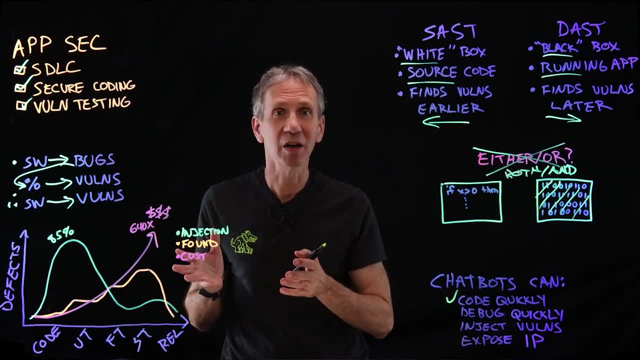 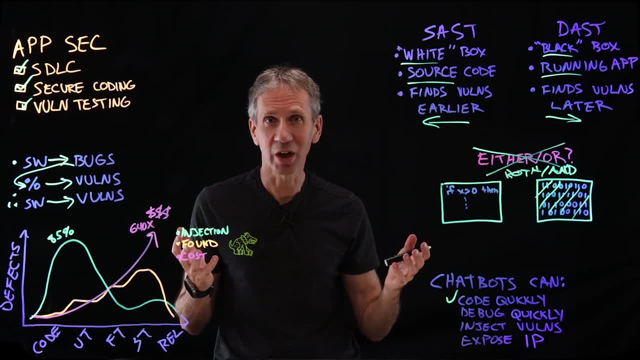 You could say: write me a routine in, say Python, that will find all the ways to make change for a dollar, and it will spit it right out just like that. So that's a nice feature that you can have the chatbot write code for you. It can also debug code. So if I've got stuck, 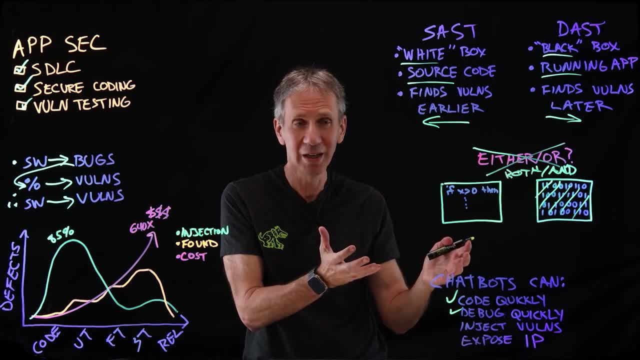 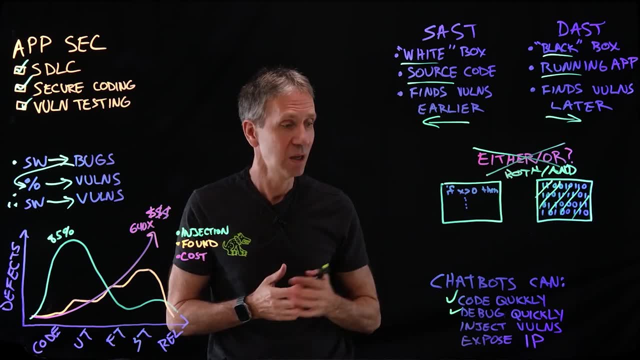 at some point during the development of some routine. I could send it into a chatbot and maybe it will find what my vulnerability is or what the bug is that I'm trying to deal with. So that's all good stuff. However, there's a downside. The downside is it could also 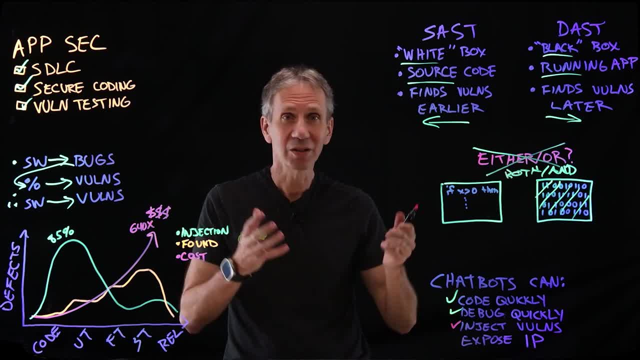 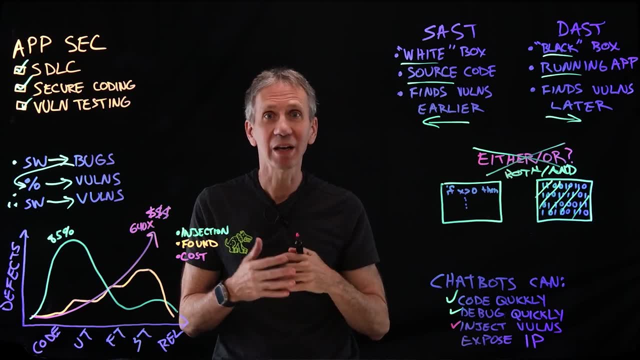 potentially inject vulnerabilities. So that is when we get source code back. we could inspect that. but probably you went to the chatbot because you had a lot of code. you wanted it to write for you, Not just the chatbot, Not just 12 lines of code, because that you could have done on your own. So are you going? 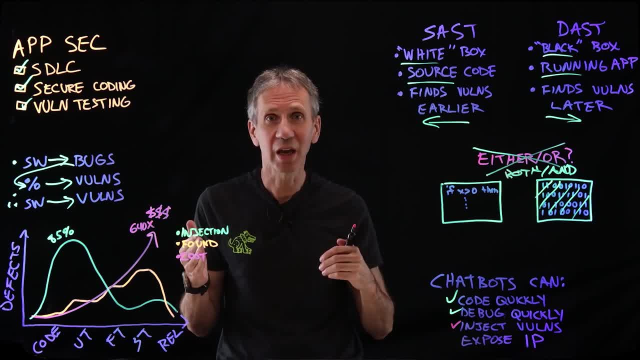 to inspect all of that and make sure that the chatbot either didn't make a mistake that introduces a vulnerability, or maybe it's been engineered in a way or someone has hacked it and it's intentionally putting a backdoor in so that all of your data is shared out. 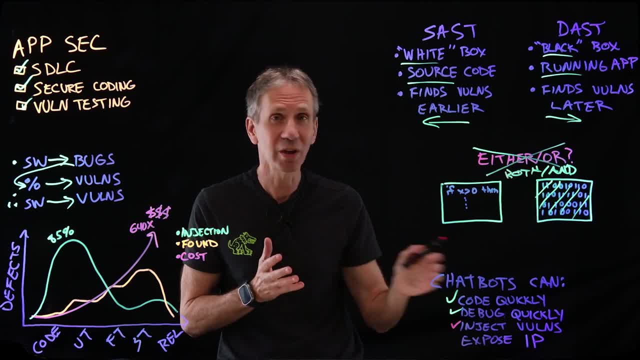 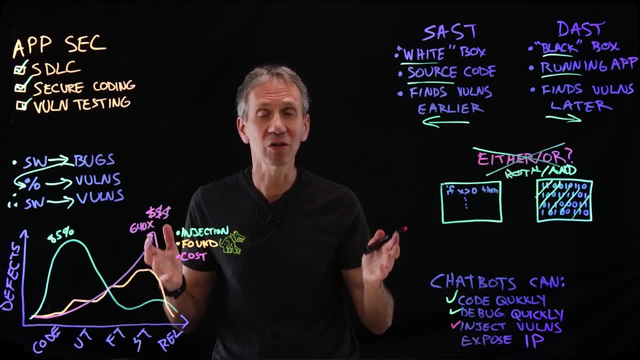 with someone else or that malware is introduced without your knowledge, So that's a big risk. It's not necessarily a trusted source like an open source library where we've had potentially thousands of eyes looking at it. In this case, it just came right straight from the source and now you're putting it. 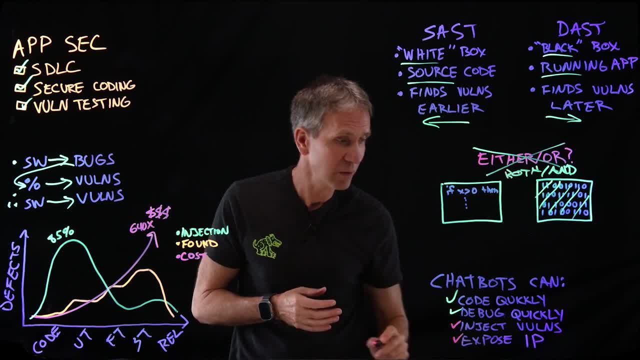 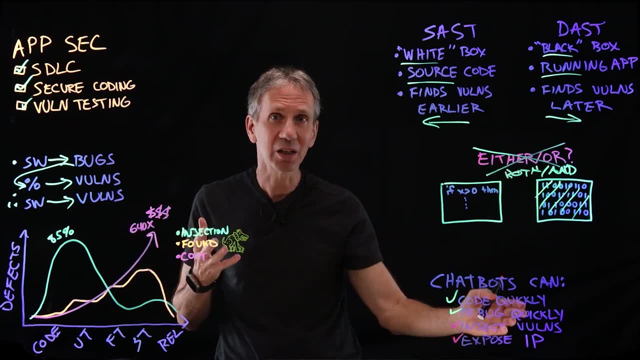 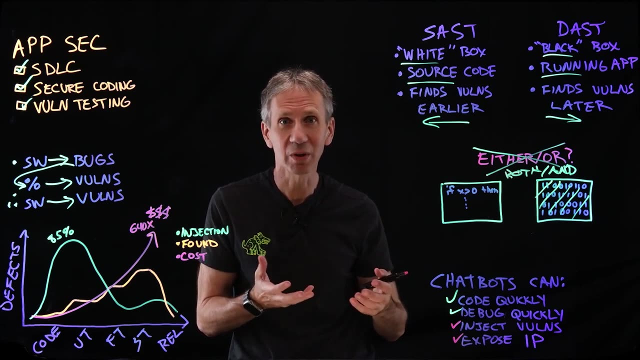 right into your code. So there's a big risk there. And another thing is: if I'm using it to do debugging, then that means I'm feeding my source code into this system and this system might expose intellectual property. If this code I have is considered a confidential, if it's a trade secret, if it's something, 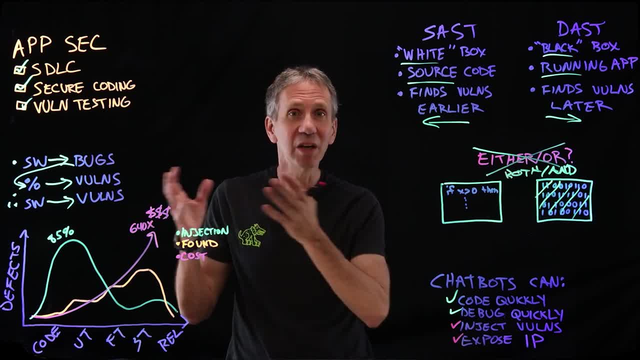 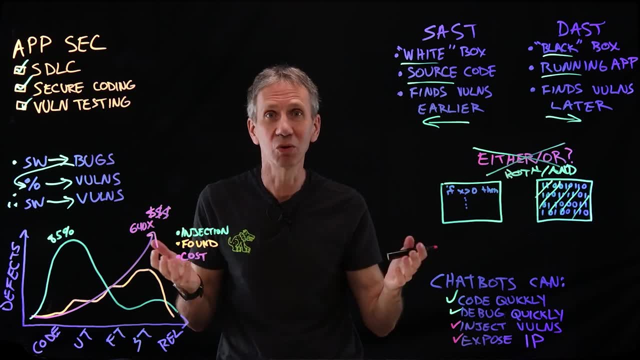 that we might copyright. Now I've just taken that and I've given it directly to what is essentially to the internet, Because it can now take that information and learn on it. It might use it. It might reuse your code in some other case. There was one major company that in fact had that. 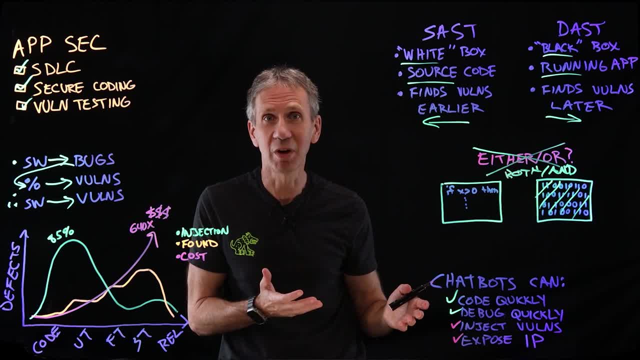 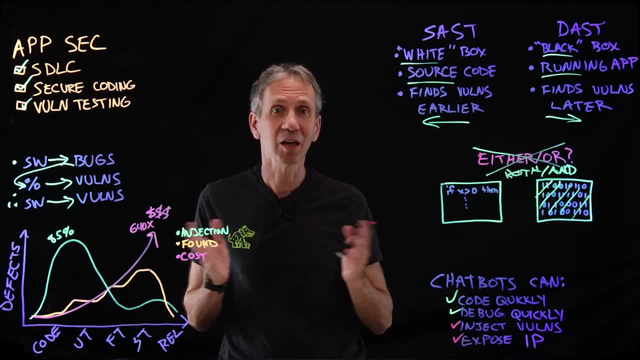 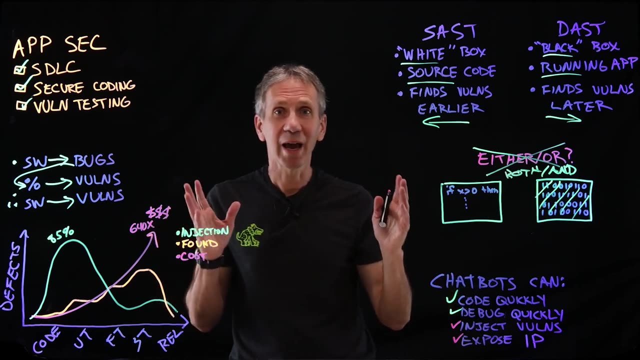 happen to them where their developers were using a chatbot to do debugging and it turned out they were releasing their proprietary source code into the system and the company decided that's not really what we want to be doing, So we need to stop that. Okay, so that's a quick look at application security. What we've tried to cover are ways 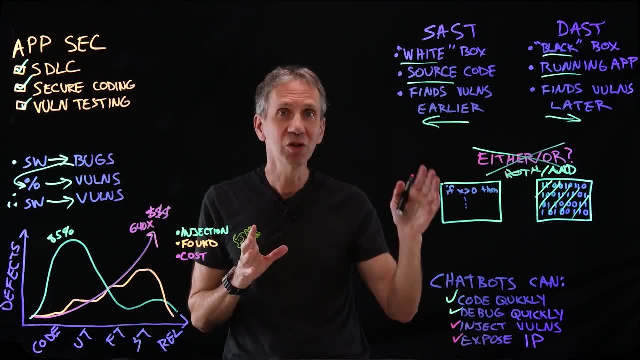 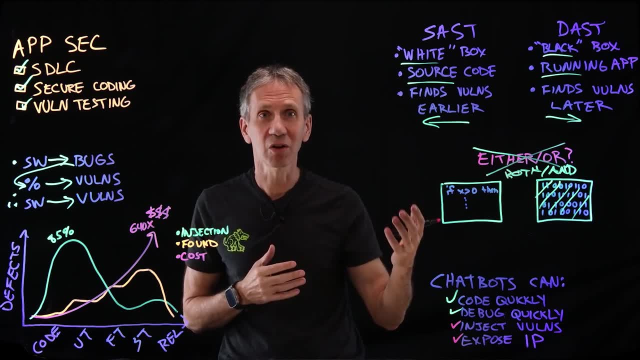 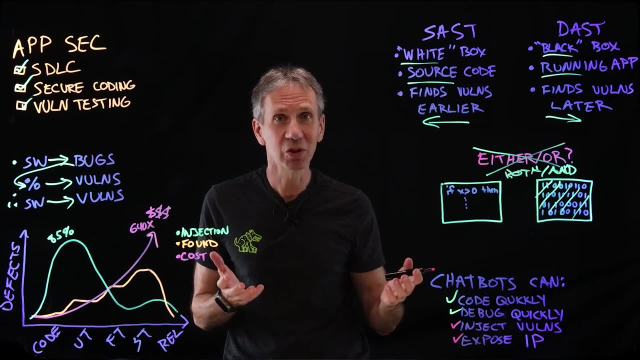 to do that Introduce process, Do a more continuous process and use tooling in order to improve the security of our systems and leverage the best of the learning from sources like OWASP, so that we don't keep making the same mistakes over and over again. It feels a lot if you've